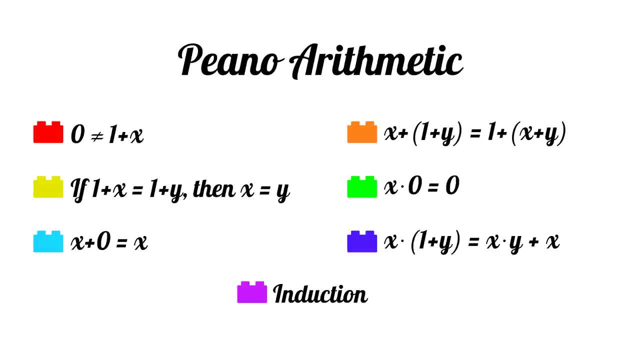 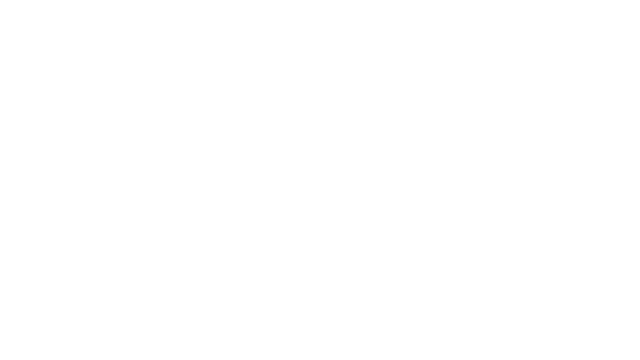 multiplication and something called induction, which we'll talk about in a future video. Putting these simple axioms together allows for a powerful look of arithmetic on the natural numbers. So what properties would we like for our own math system? Well, we'd like it to be powerful enough to be interesting, so we say we want it to be. 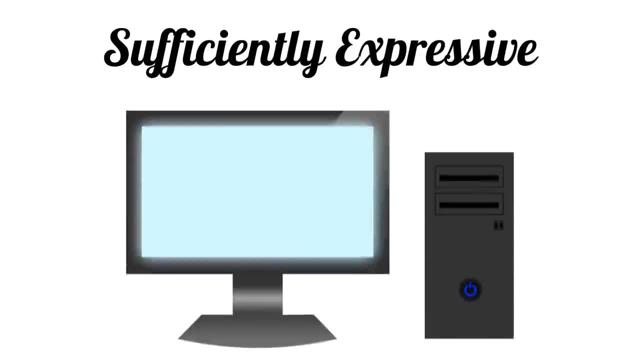 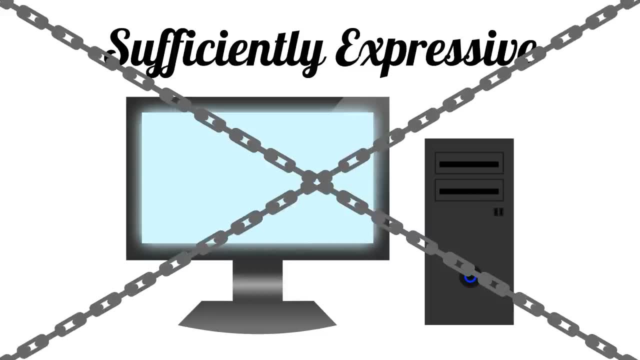 sufficiently expressive or strong enough to describe computation. Given how complex our technology has become, this may sound pretty restrictive, but it's not. A system doesn't need too much to describe computation. It's just a simple axiom that can be used to describe a. 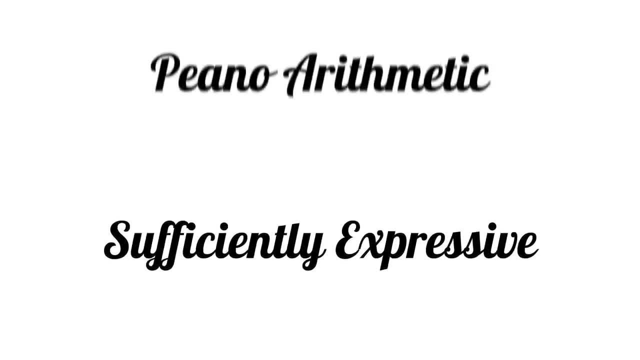 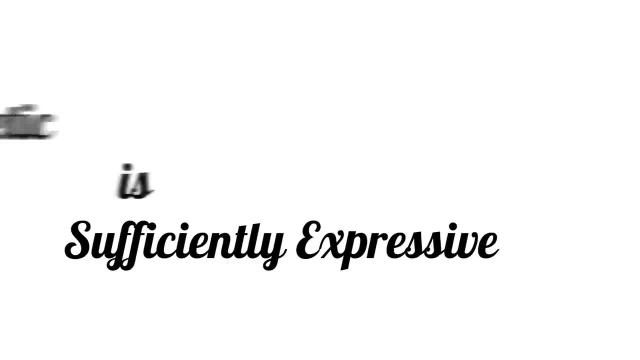 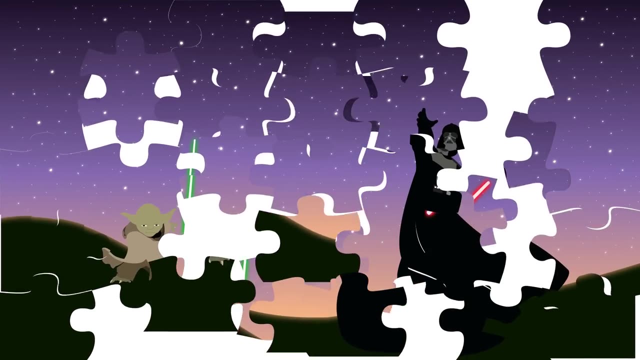 computer program. Even a simple system like piano arithmetic, which we just discussed, is sufficiently expressive. Another property we might like is the ability to prove every true statement. This is known as completeness. We would like math and science to answer all of the unknown. 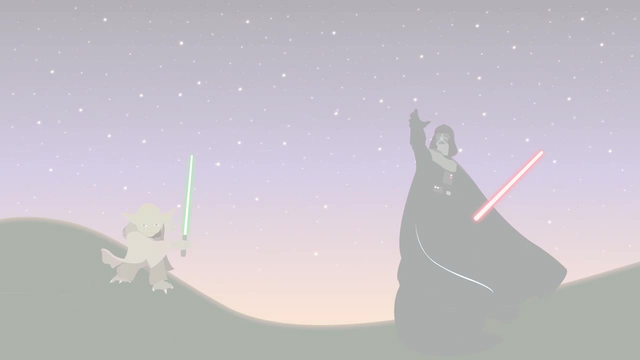 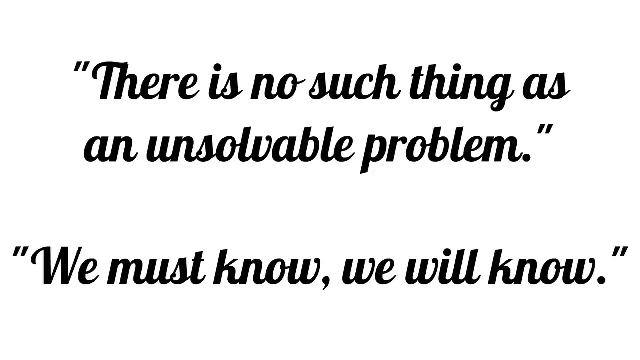 questions that we're still exploring. As mathematician David Hilbert said, there is no such thing as an unsolvable problem, and we must know, we will know. It would be great if our system could prove everything that is true within it. 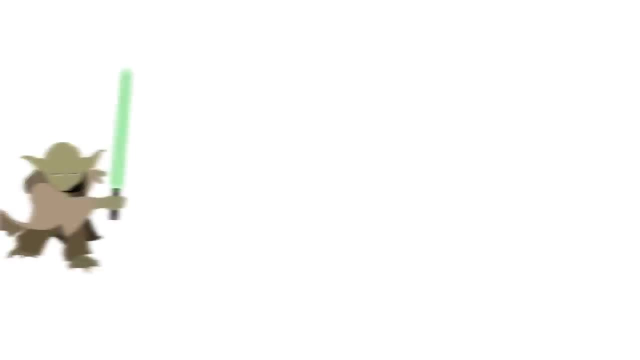 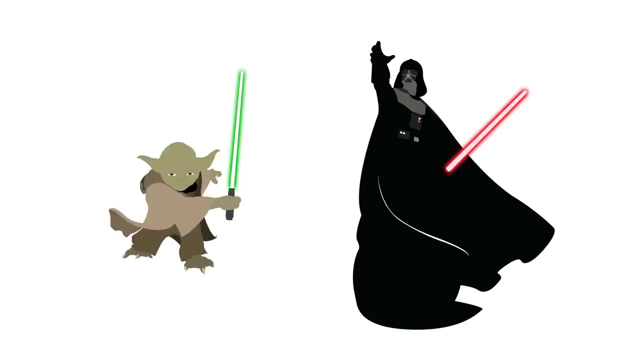 One final property we might like is that if we can prove something, we shouldn't be able to prove the opposite of that thing. Being able to prove a statement and its opposite would mean that we would be able to prove false statements, since one must be true. 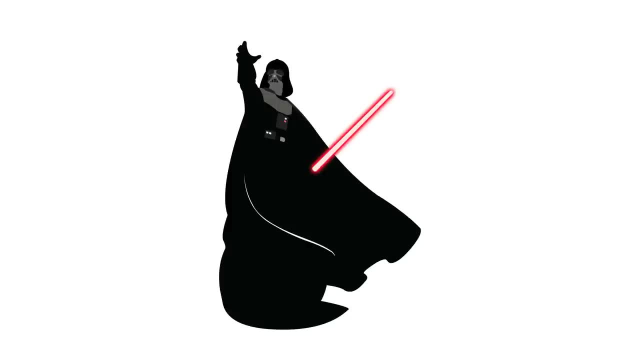 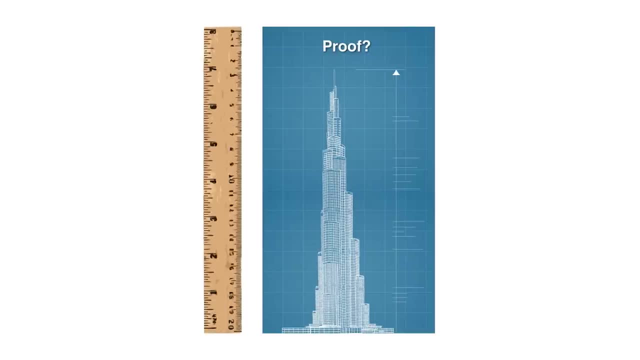 and the other false. If we could prove false statements, we would have to question all of our mathematical proofs, since they could lead us to an incorrect conclusion. If you're ruled by a ruler, any measurement made with that ruler would be untrustworthy, Proving at most one of a 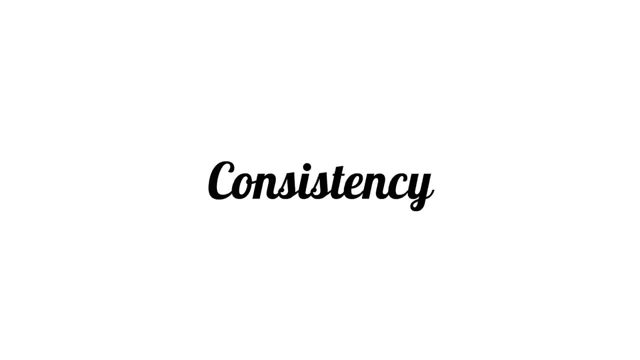 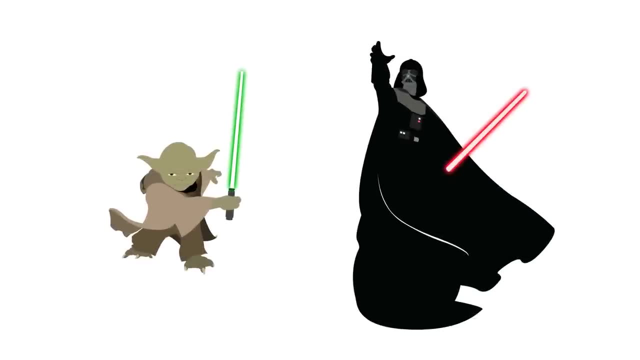 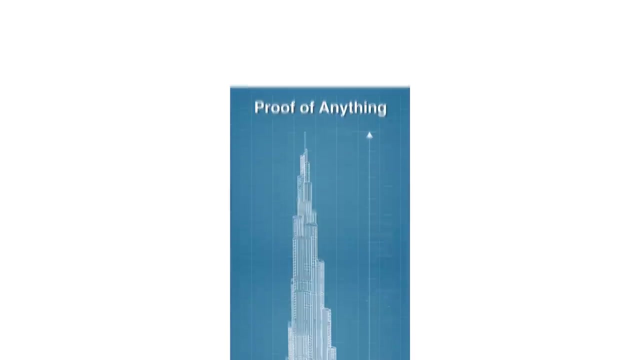 statement and its opposite is known as consistency and seems like a no-brainer. However, an inconsistent system might be worse than it looks at first glance. This is because an inconsistent system can prove anything. To understand why this is, let's say that our system is inconsistent and can prove, for example, both there are flying. 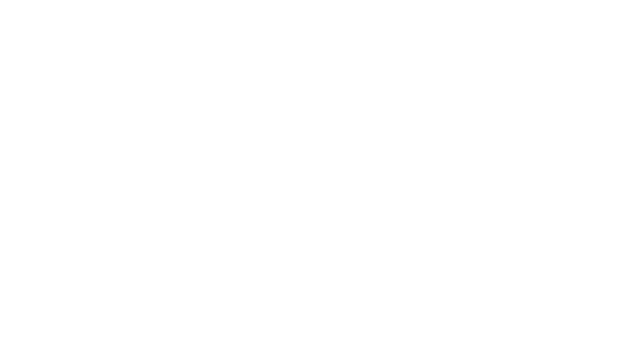 pigs and no pigs can fly. Now let's try to prove some random statement such as unicorns exist. The statement there are flying pigs or unicorns exist must be true, because we can prove that there are flying pigs making the full or claim true. However, we also know the statement there. 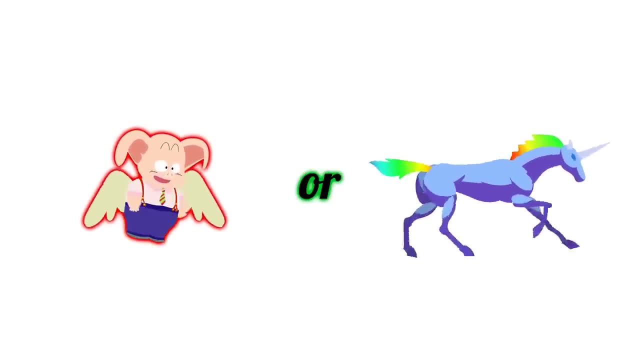 are flying pigs is false because we can prove that pigs can't fly, The full claim must still be true because we've already proved it. For the claim to still be true when pigs can't fly, it must be the case that unicorns exist. We could have replaced: unicorns exist to prove. 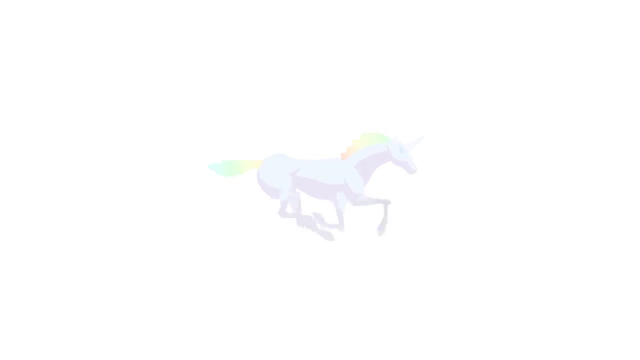 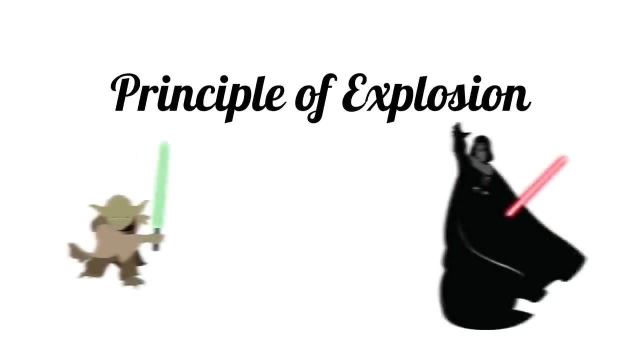 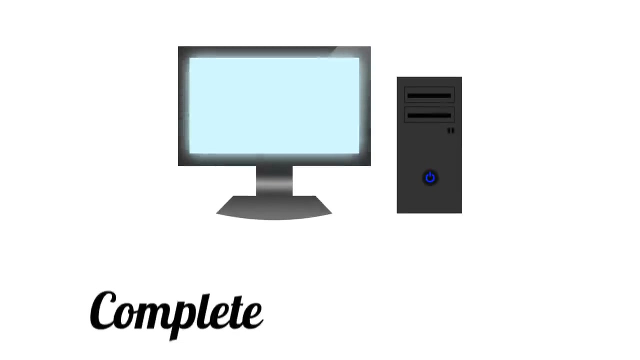 anything we wanted, including unicorns, don't exist. This is known as the principle of explosion and is one of the reasons why we definitely do not want an inconsistent system. So far, we have a sufficiently expressive math system that we want to be complete and consistent. Unfortunately, this isn't possible. 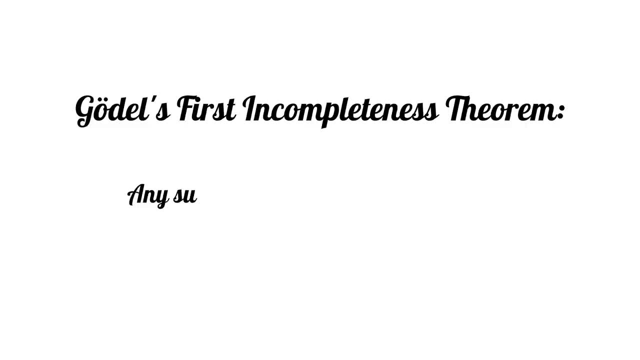 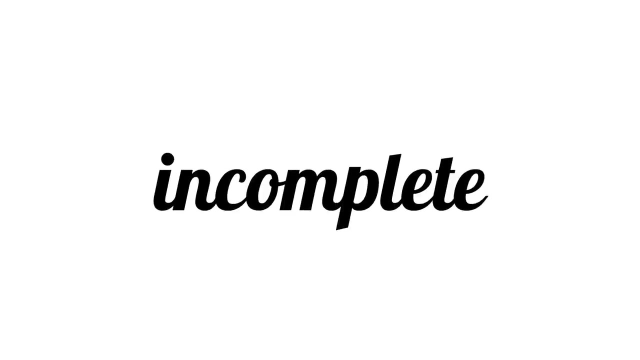 Gödel's first incompleteness theorem tells us that any sufficiently expressive math system must be either incomplete or inconsistent. This is very unfortunate news and given how bad inconsistency is, we're forced to hope that our system is incomplete. You might think that it's okay for our system to be incomplete. We can just add any unprovable. 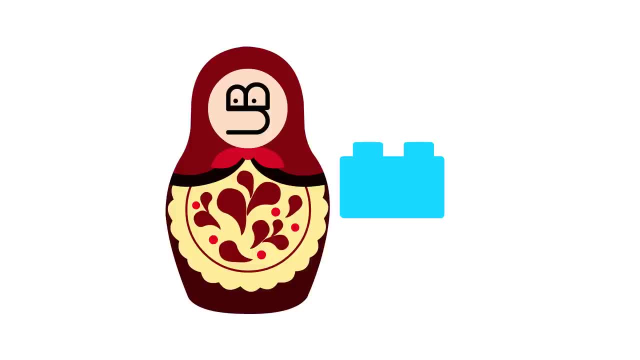 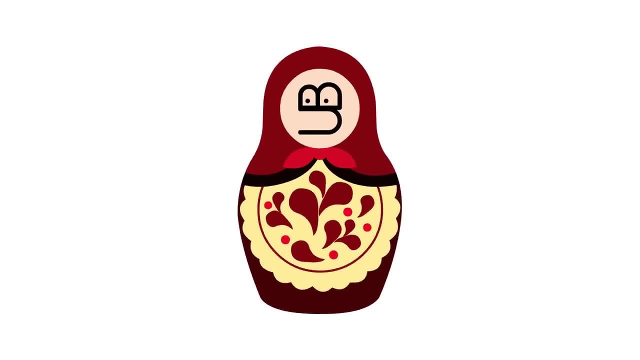 statement as an axiom and call it a day. Unfortunately, this doesn't quite work, because adding a new axiom like that actually creates a brand new system, and this new system is still susceptible to the incompleteness theorem, meaning that there will 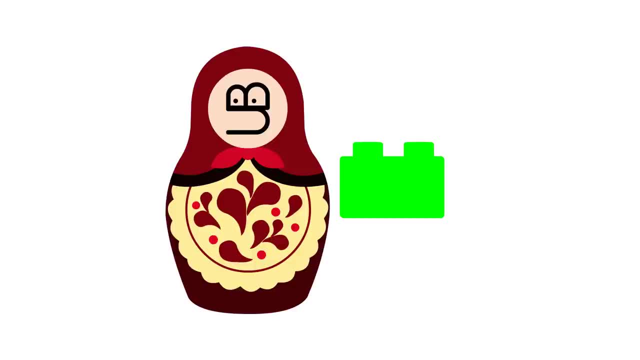 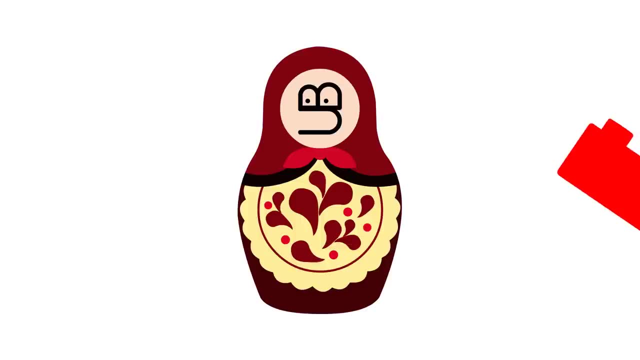 still be some true statement that we can't prove. in this new system, We can keep adding these unprovable axioms, but there will always be another one lurking behind the corner, Forced to accept the incompleteness of our system. let's turn back the 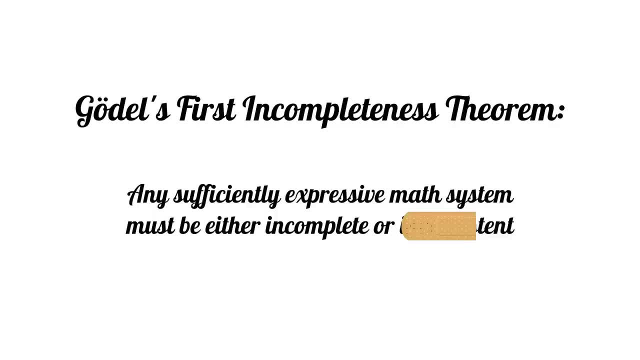 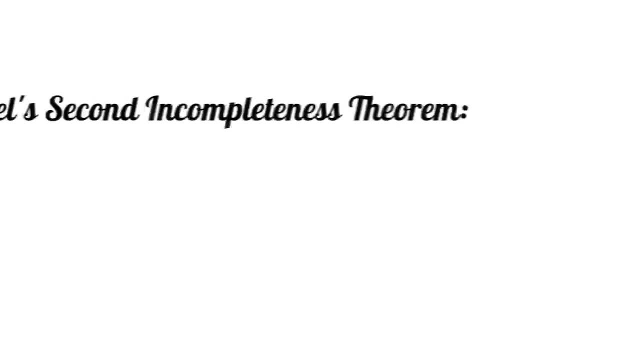 to consistency. We would like to patch that hole at least. so let's prove that our system is consistent for peace of mind. Unfortunately, again, Gödel's second incompleteness theorem tells us that a consistent math system cannot prove its own consistency. We really need our system to.